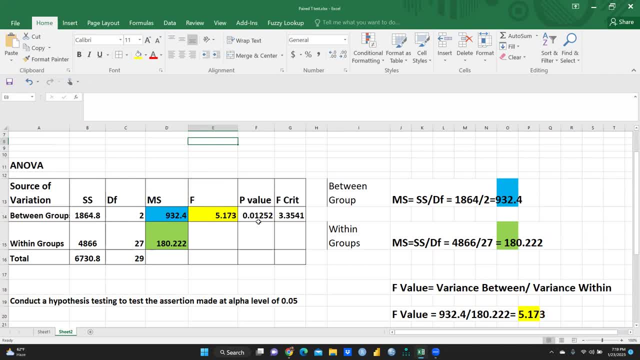 5.173,. P value 0.012,. F critical 3.35.. That is summary already When we talk about within the group 4866, S's value degree of freedom 27,. MS 180.22,. 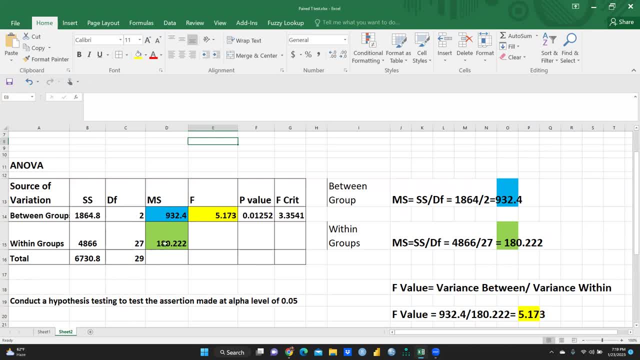 and F is already. I mean, with the help of both these values, we had calculated F. I had already prepared a detailed video on ANOVA, One-way ANOVA, So I am going to give this video link in my description. 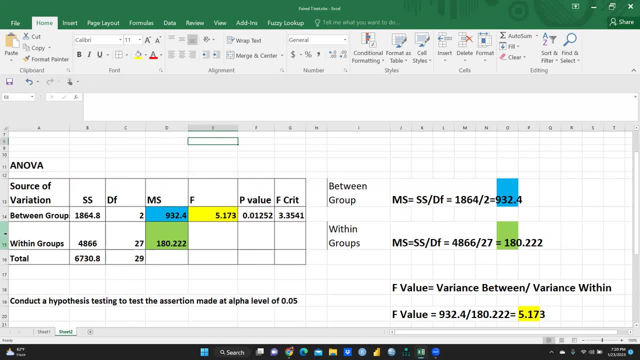 In my description box you can go through that particular video. But here is in this video I am covering only how we are going to interpret these results. So how come we have reached on this particular value? So see thing is there between the group. 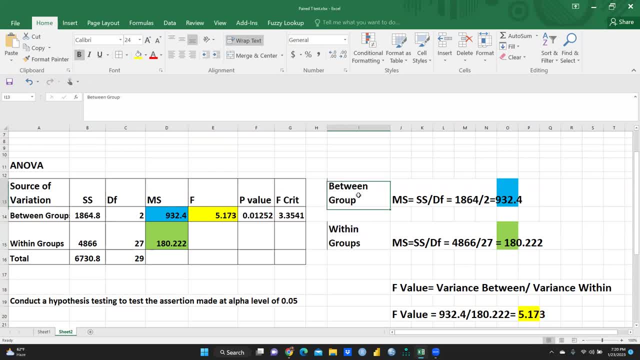 you can see here and within the group, you can see here, between the group MS, how we are going to calculate, How come we have to reach on this particular value, 932.4? Okay, Okay. So first of all, what we have to do: 1864.8 divided by 2.. 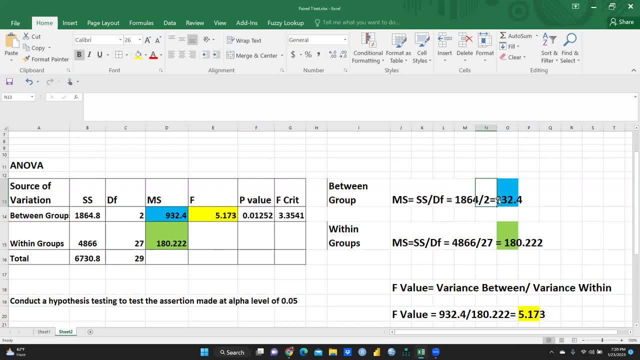 1.68 divided by 2.. So let me check here. I'm just putting formula here And this value is divided by this value, And what is the answer? So answer is same: 932.4.. Because I have not taken into consideration. 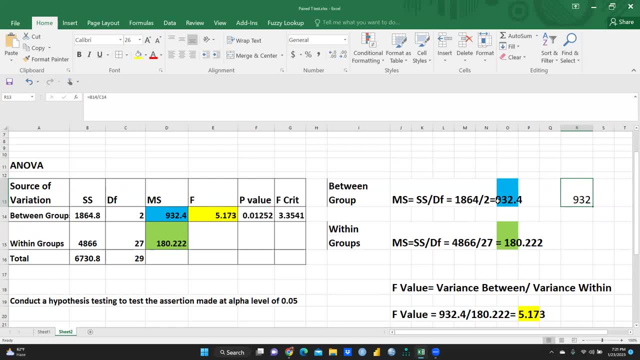 0.8.. So here is 932.. Same answer, MS. we had calculated. So you know, you understand this value. How come we will reach on this value? Then we come to the within the group. Within the group. same thing we are going to apply here. 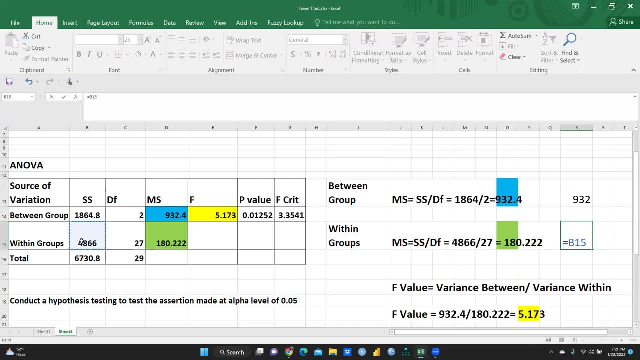 I'm just putting formula here: This value, right, And that is divided by this, divided by this value. Let me clear this: This value divided by this value. Let me clear this, This value divided by this value, And enter So 180,. you can see here: 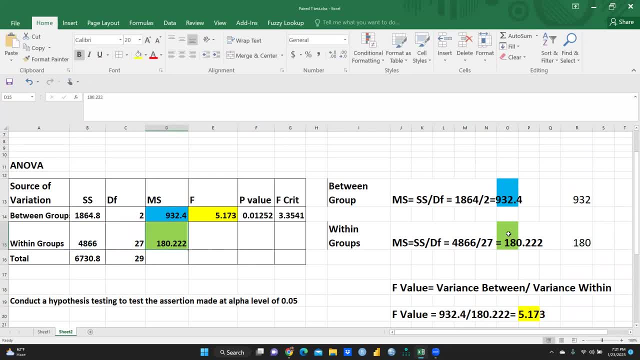 Same answer we have got Right Now how I will reach on this particular point. F factor, F ratio And F value is variance between divided by variance within. So variance between here is, you can see here, between the group, this value and within the 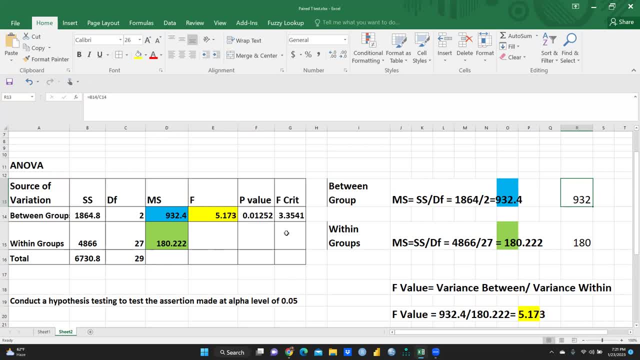 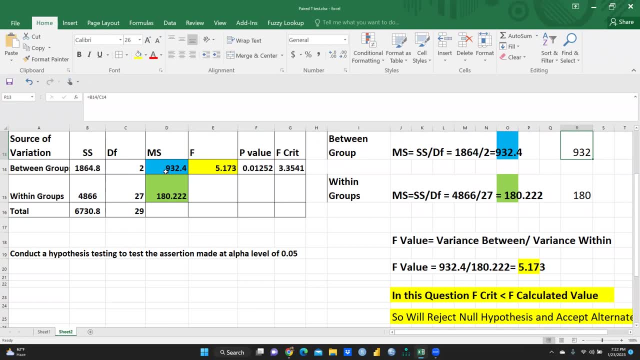 group this value. So I'm just putting this value. So variance between here is, you can see here, between the group this value and within the group this value. So I am just putting formula here, I am just putting within. here is the variance between: 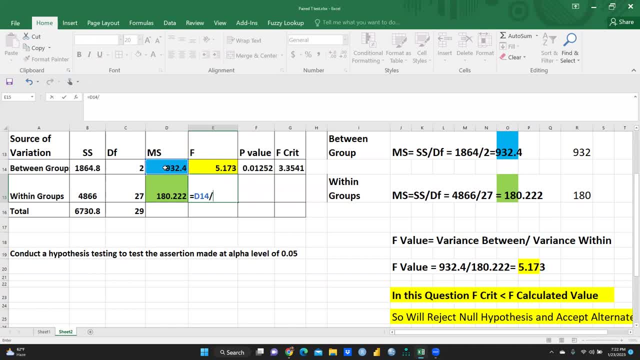 So this is my variance between the group. I have put it this: selected this cell divided by within the group And let me press enter. So I am sure, same answer, we have got. Same answer, we have got Right. 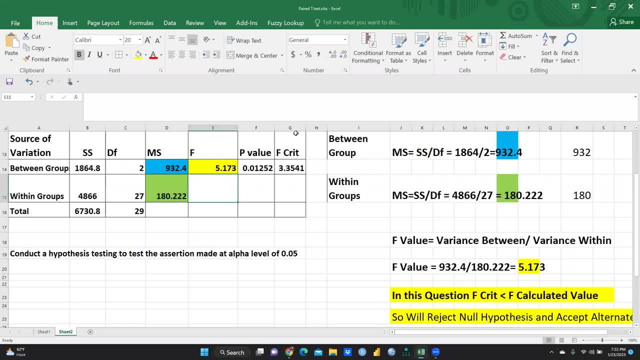 So let me clear this After that, how we will reach on F critical Now what, how we are going to interpret these results. So we would interpret these results after getting this F value. We will find out because conduct a hypothesis, because that is already given in question paper. 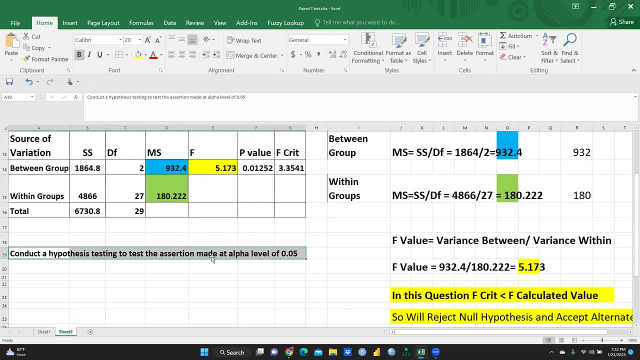 Conduct a hypothesis testing to test the assertion made at alpha level of 0.05.. Now I would like to check what is the critical value of F value. Critical value: whether it is same 3.3541.. So let's. 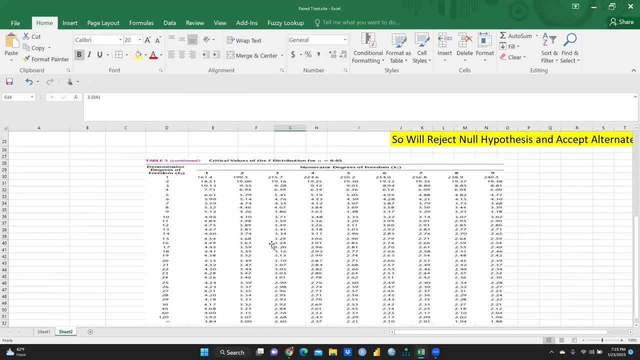 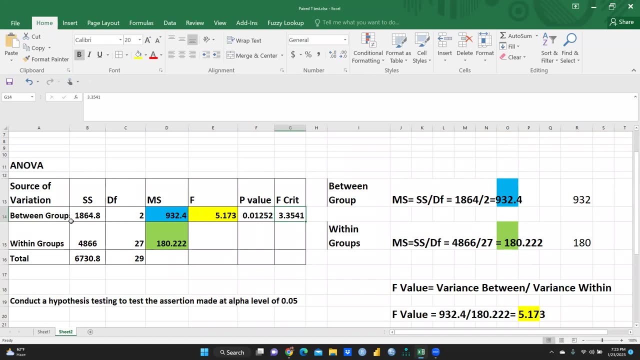 Let me check in F table. Here is you can see this is my F table. In this F table we can see here degree of freedom is already given between the group and within the group. Between the group is 2 and within the group is 27.. 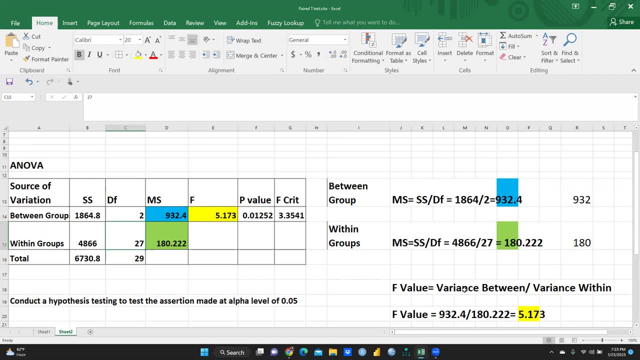 So what we have to do here is, in this formula, variance between Between, that means 2.. That means vertically we will see 2 degree of freedom And horizontally We will not. sorry, vertically we will see 27 and horizontally we will see 2, right, because 2 is our numerator and variance within is our denominator. 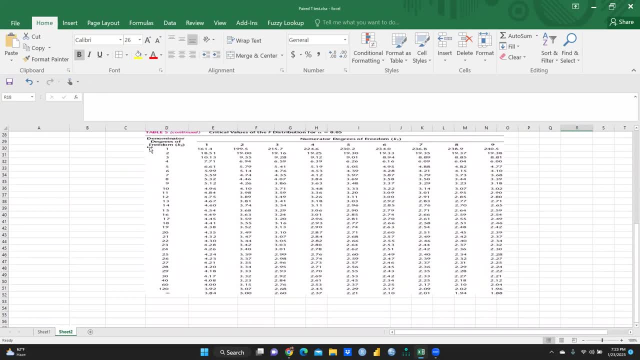 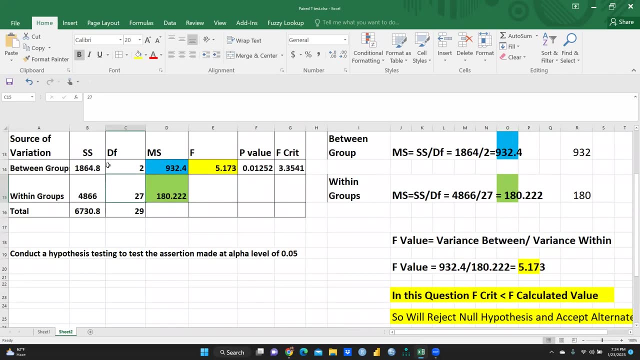 So you can see here denominator already in this table given denominator degree of freedom. So my in my question denominator degree of freedom is 27 and numerator degree of freedom is 2.. So let me check 27,. where is 27?? 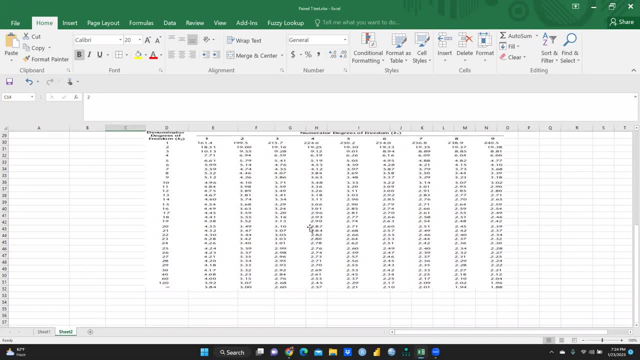 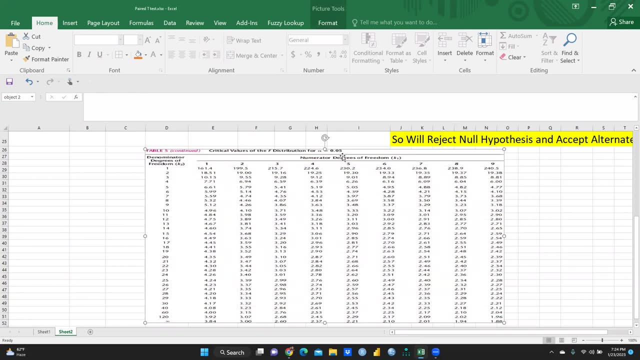 This is 27 and with 2 and is already you can see alpha value is 0.05, alpha value is 0.05, F distribution and critical value 27 is our denominator and numerator is here is 2.. So we will vertically we will see right, there is 2, right. vertically we will see 27 and horizontally 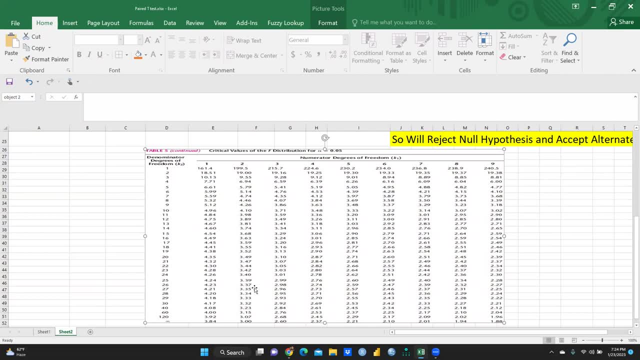 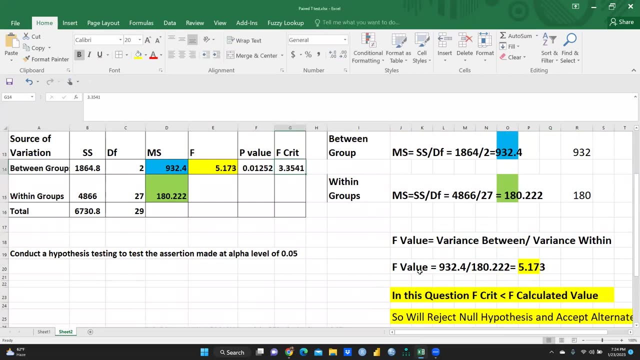 We will, We will see. 2 and 3.35 is my final answer, So my same is same is I think we are getting 3.35 critical value, So when, how we can select whether null hypothesis is rejected or accepted. 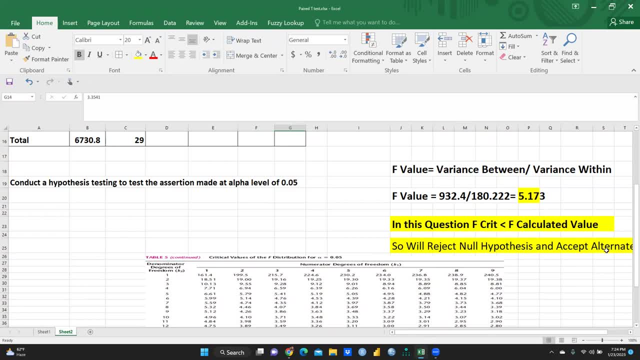 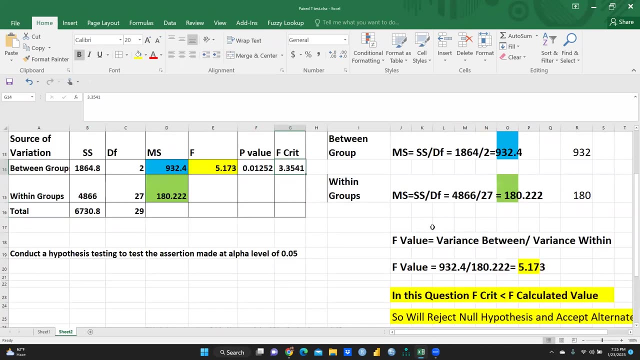 So we will reject null hypothesis and accept alternate hypothesis. Why? Because in this question F critical value is lesser than F calculated value. My F calculated value is 5.35.. So this is critical value, means tabular value, table value. it is less than my calculated value. 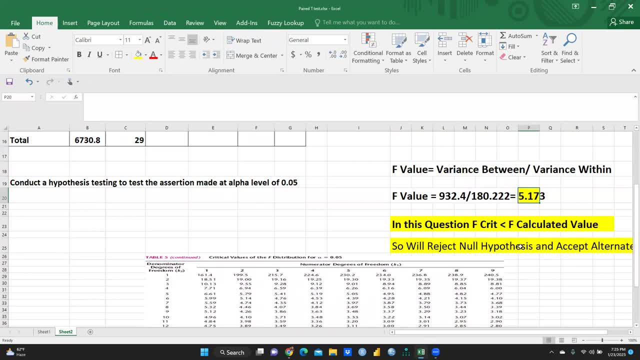 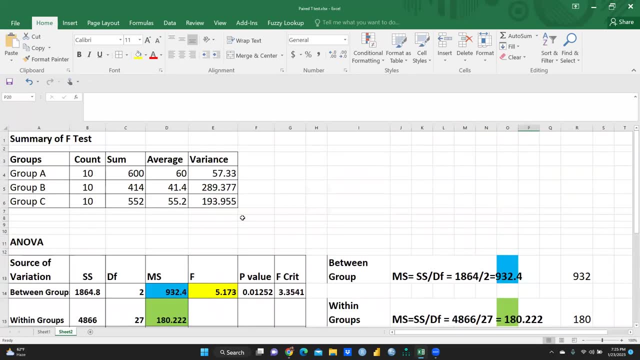 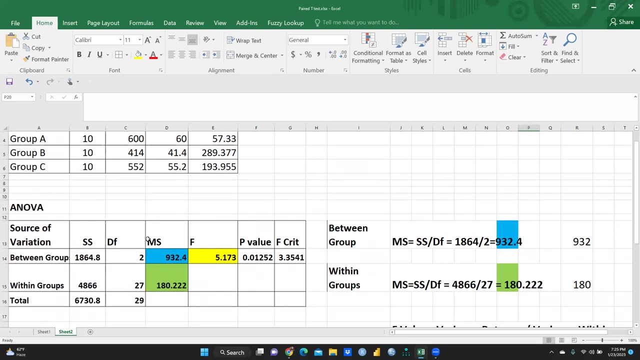 So that is why we are rejecting null hypothesis and accepting alternate hypothesis. So I hope you could be able to understand, when we are getting summary of ANOVA, how we are going to interpret these results. We can further cross Check all these things, whether we are getting the same results. 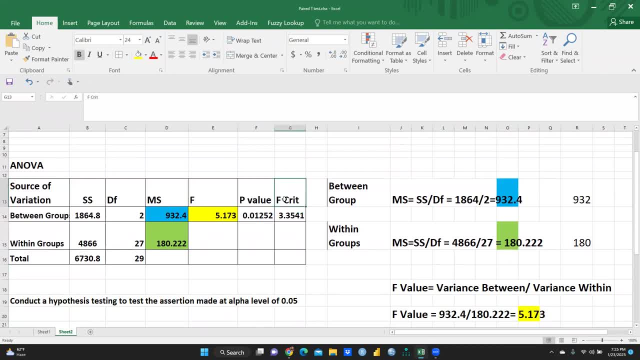 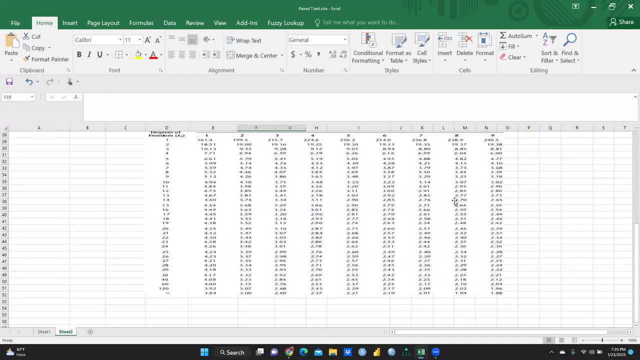 Manually. we had calculated all these things And after that F critical value we have cross-checked at the alpha level of 0.05.. We have checked in our this table, F table and critical values of F distribution. Alpha is 0.05.. 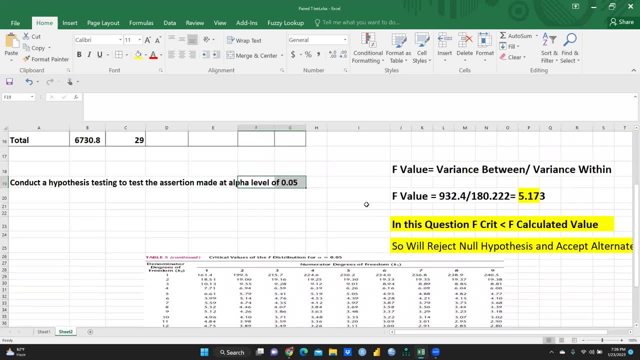 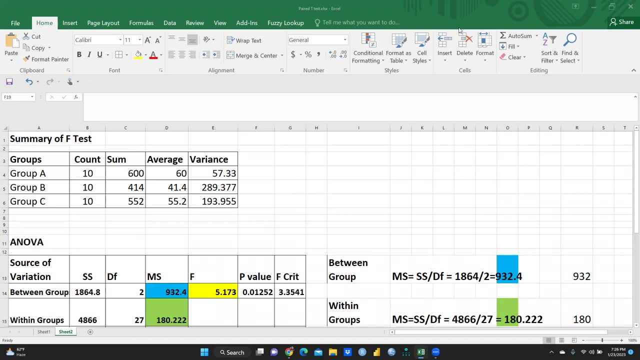 Finally we have checked and now we had written our conclusion, So I hope this video would be helpful. Thank you, Keep watching, And I am giving you in my description box earlier recording detailed video on ANOVA- one-way ANOVA. Thank you.